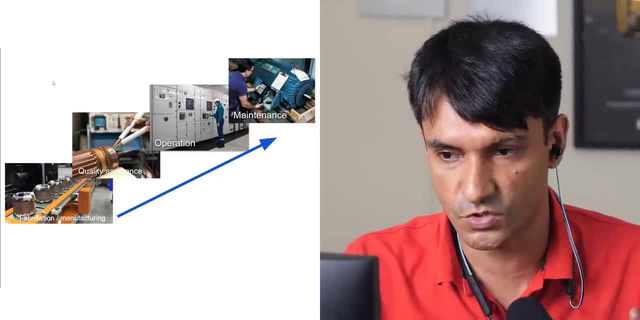 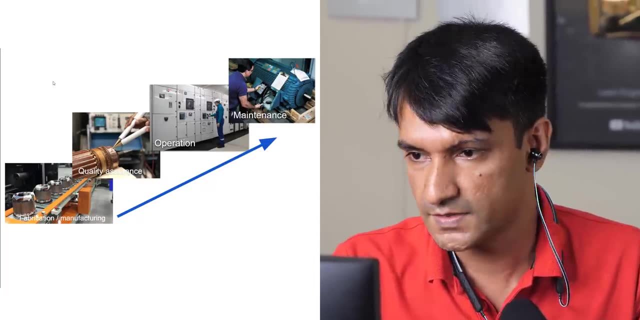 Somebody will make sure that motor is working perfectly well, It is producing sufficient torque And the current values are right. Once the quality assurance is done, when the motor is ready, somebody will buy it. Then that person will use it for many years or many months. 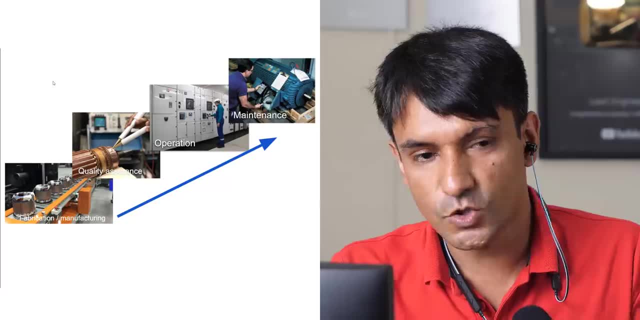 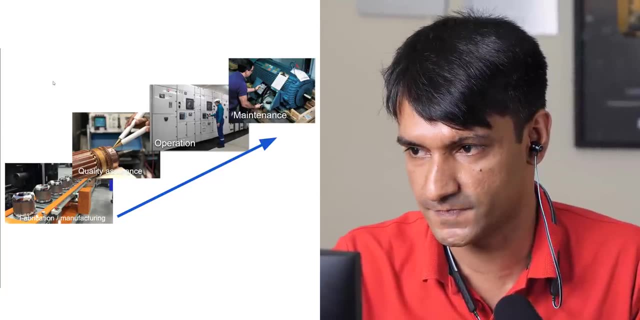 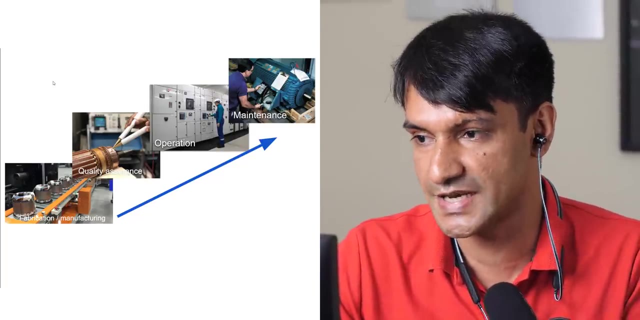 That is operation. And during this operation, maybe after 12 months or many years, the motor may break down. Then it has to go for maintenance purpose. Right, So these are four different stages of an electric motor, Four different stages in an electric motor's life. 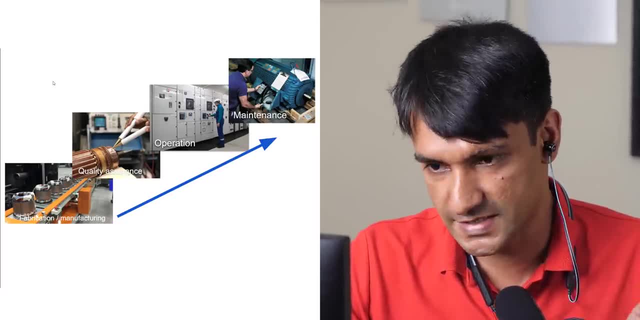 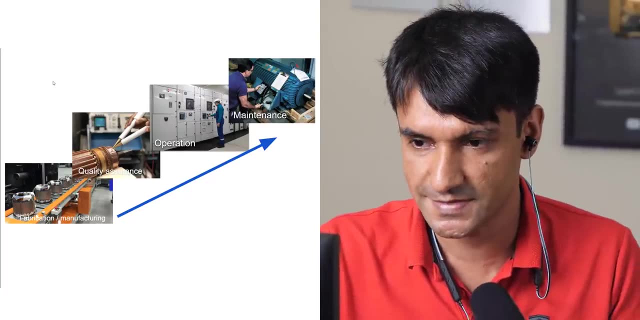 And the interesting thing is that the motor is not just a motor. The interesting thing is that behind all these stages, there should be an engineer to do this work. Here, in this fabrication stage, we will call him fabrication engineer. In this quality stage, obviously, quality assurance engineer. 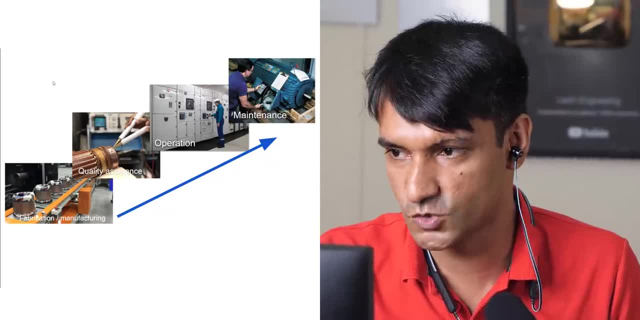 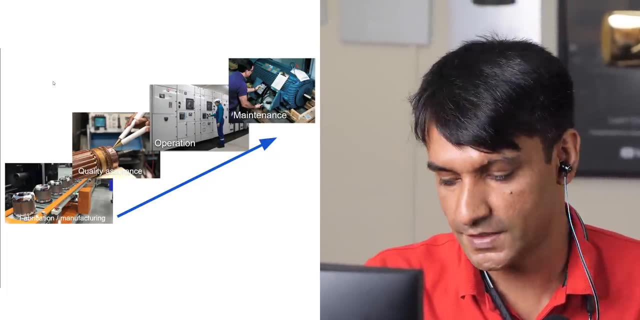 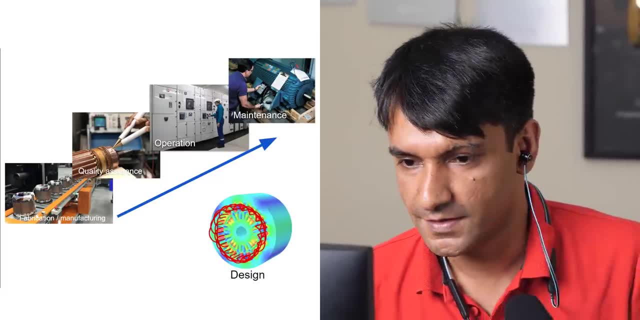 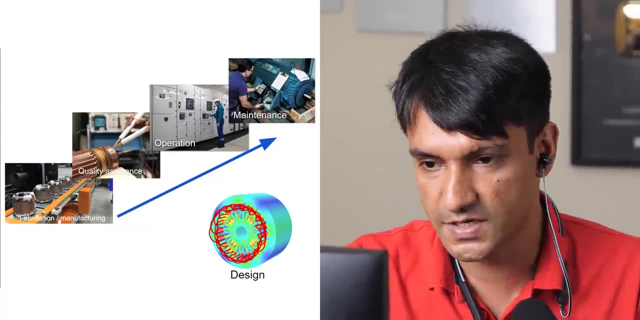 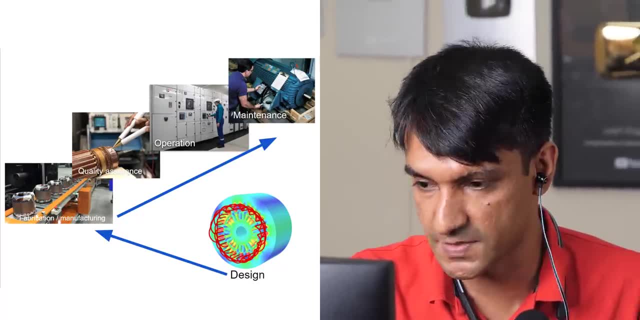 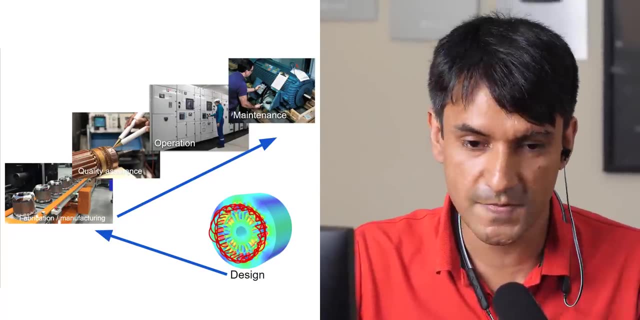 In the design stage, there was a design team Especially for an electric motor, a big design team. They had a vision, They had a dream, They had an objective. They designed a motor. By design what I mean? they designed exact number of slots, number of turns needed for. 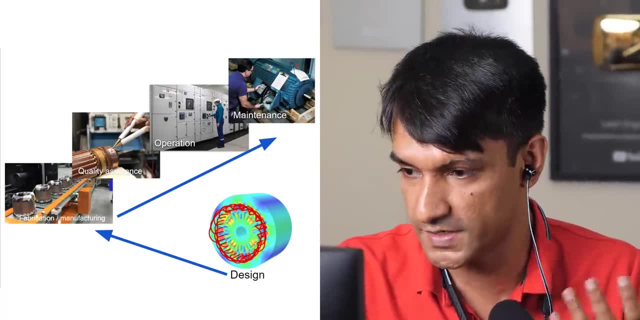 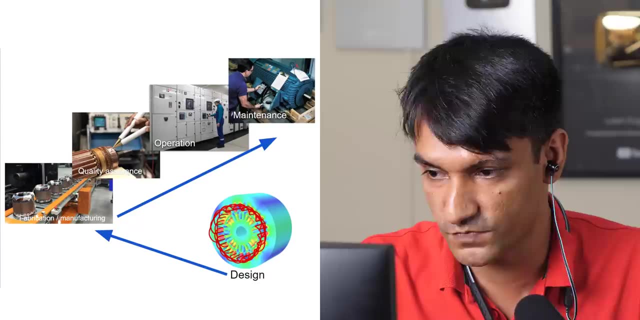 the motor and how much torque it will produce at the peak rpm, what will be the peak efficiency and what is the torque curve? or even how much temperature, what will temperature of the motor when the at the highest load? all these things they are predicting, they are designing, they are. 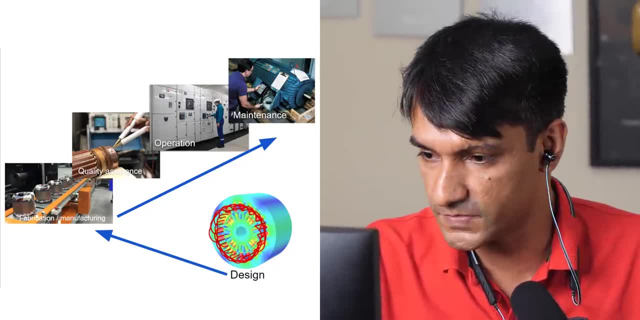 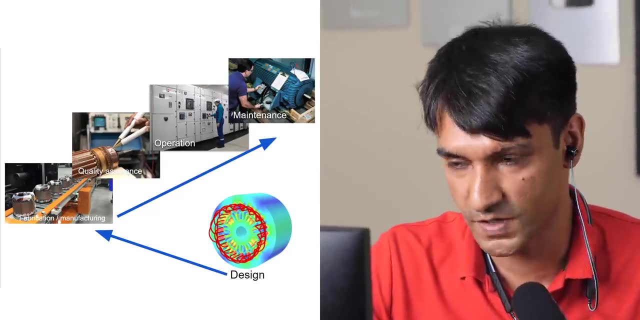 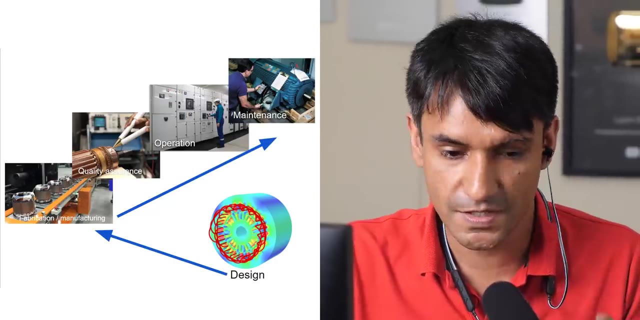 calculating. they are redesigning it. so this is a big task. only after the design stage is complete, when the design is final, it's most for fabrication and the remaining operations. so obviously you need a huge amount of subject knowledge in design field. without subject knowledge you'll be a complete failure. so if one of your seniors are saying that, 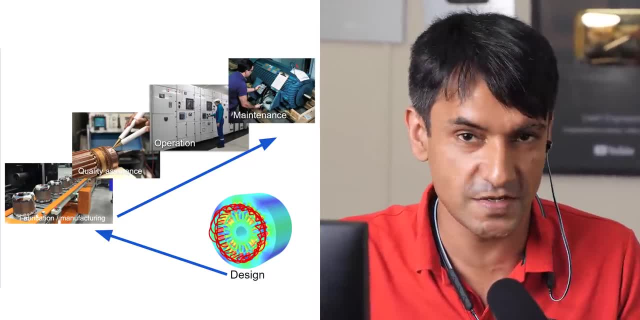 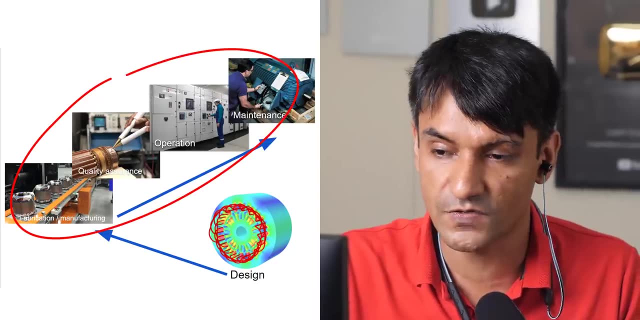 engineering is all about core engineering is all about practical experience, the subject knowledge, the mathematics you'll learn they have no use. then you can obviously guess that they are working one of these four areas not in design field, because if you're a design engineer and if you 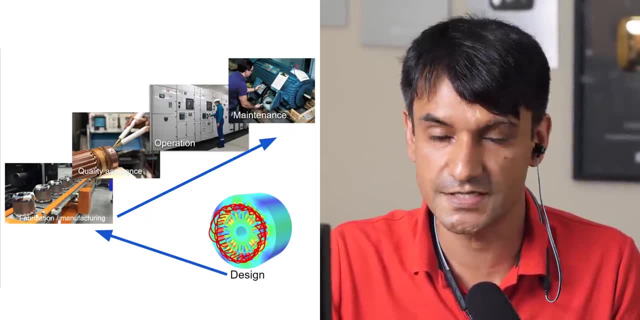 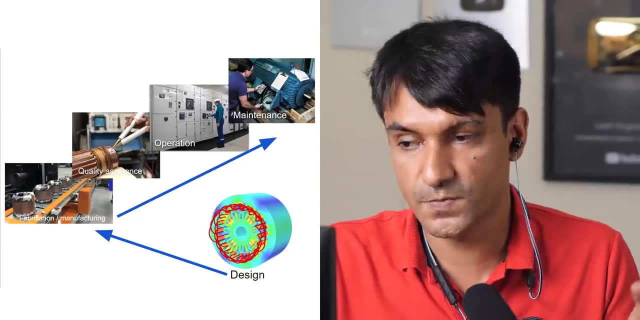 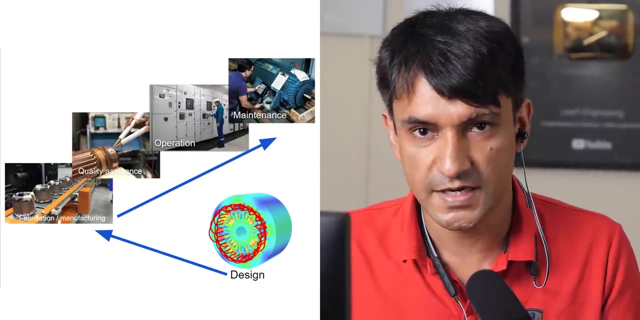 don't have subject knowledge, you are going to be failed. failure it's just not possible without subject knowledge. so a design engineer- in this case they- have innovated a motor right from a scratch. from an idea, they built a motor, but that's. that's not the case always. a design engineer can innovate a product, that's true, but most 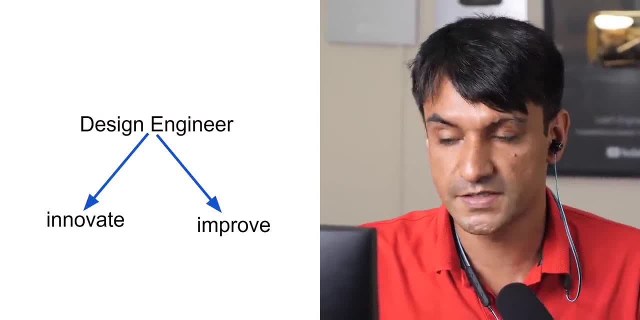 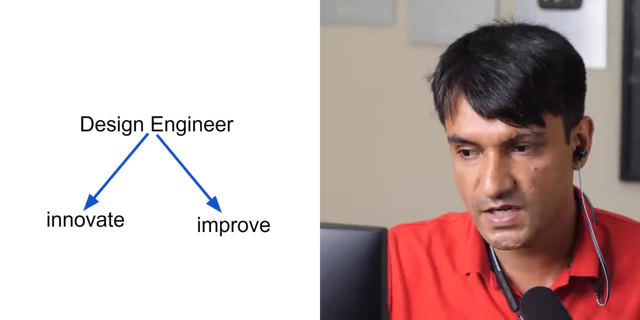 of the time, they will be improving a design. that's the case most of the time. nowadays, they can innovate, they can make a new product from scratch. that's obviously fine, but most of the time what happens in big companies is all about improvements, even minor improvements. take a steam turbine. the engineers 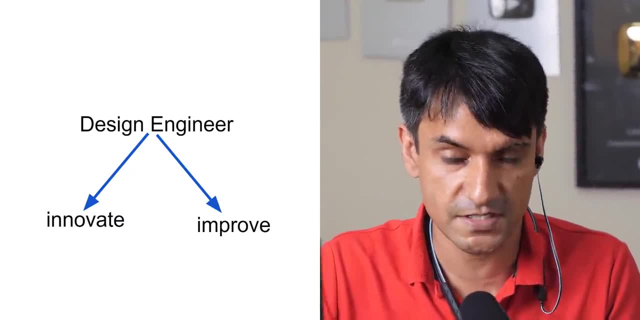 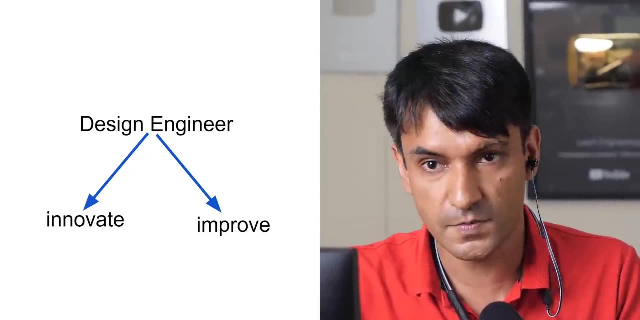 will try to improve the efficiency by- maybe by 0.1 percentage. that's a big deal. or take an ic engine and try to reduce the pollution developed by 0.5 percentage. or a motor: reduce the weight of the motor and still maintain the same torque output. that's a big achievement. material savings and 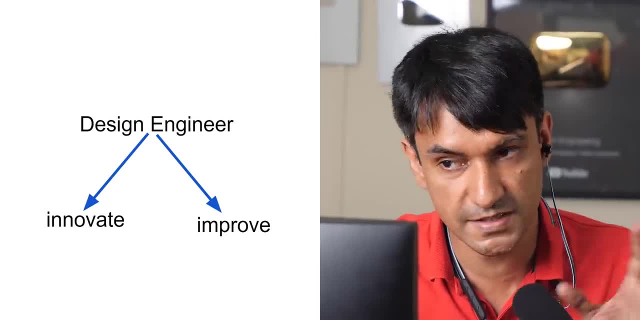 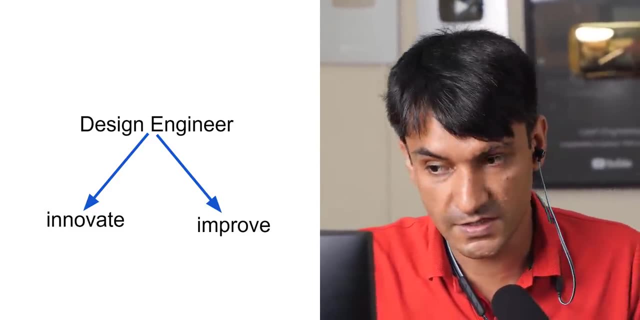 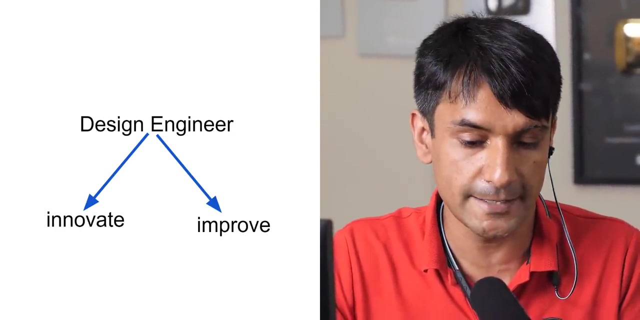 money saving. so most of the time a design engineers in big companies, established companies, will be working on improvements, design improvements rather than a new design or innovation. but even here for improvements you need a deep subject knowledge and understanding of the technology or physics behind that. without that you will be like a car without any proper guidance, it won't reach anywhere with just. 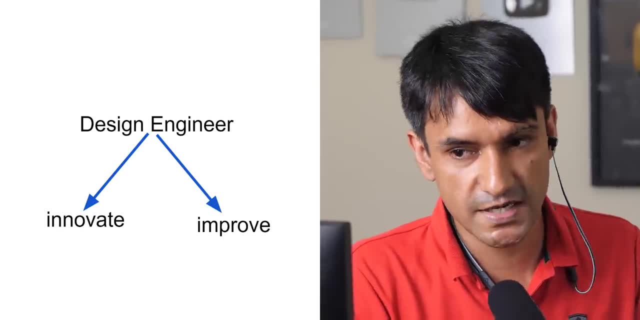 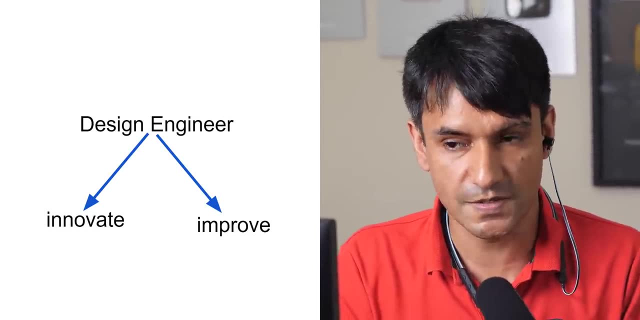 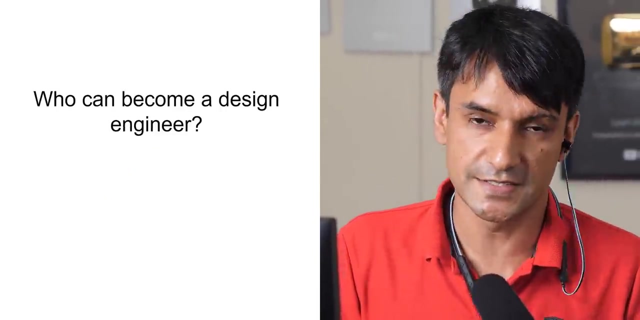 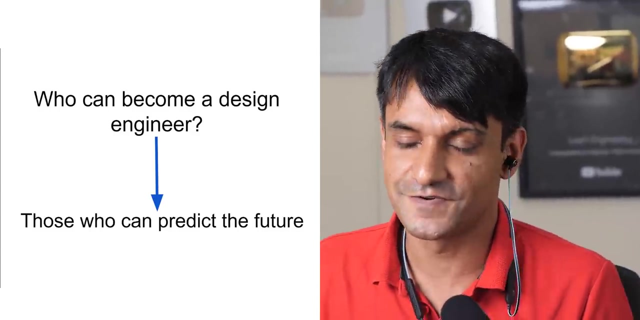 trial and error. so we understood. a design engineer means the subject is very imperative. you cannot, you can't, be a good engineer without proper subject knowledge. now the next big question: who can become a design engineer? the simple answer is that those who can predict the future. a funny answer, right, but I will. I will prove this. I will. 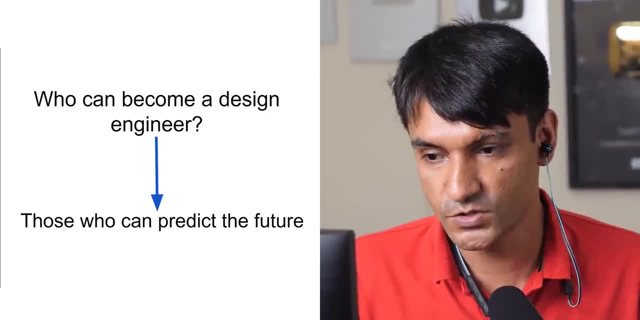 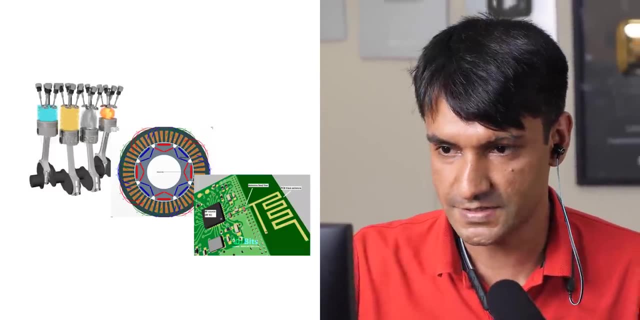 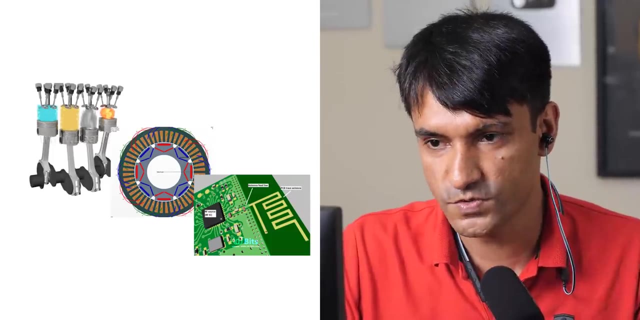 prove why this funny answer is right. you, with help of some examples, why those who can predict the future can become a design engineer. check this three example from three different branches of engineering. take this petrol engine. so if you are someone, what will happen to this motor engine's torque output if I? 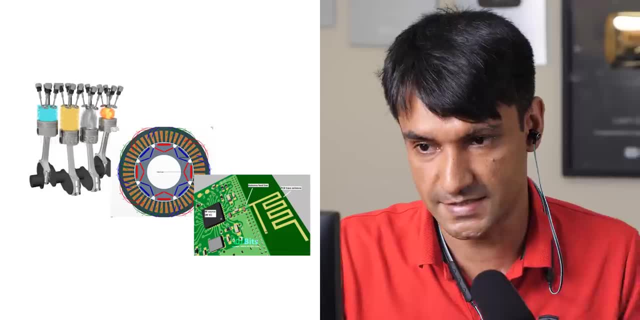 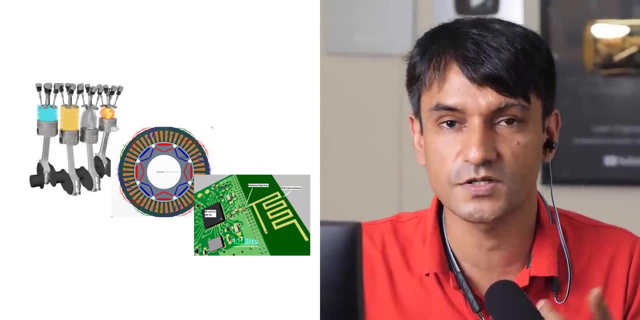 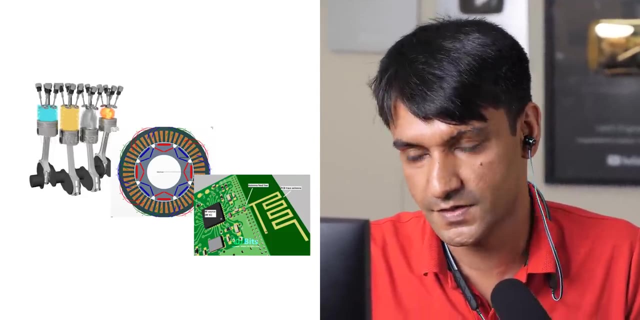 increase length of this connecting rod. can they predict it? this engine is a working engine is working fine. but if I change the length of this connecting rod, what will happen to this torque output? if somebody can give a good answer logically, he can be a good design engineer for IC engine field. or take 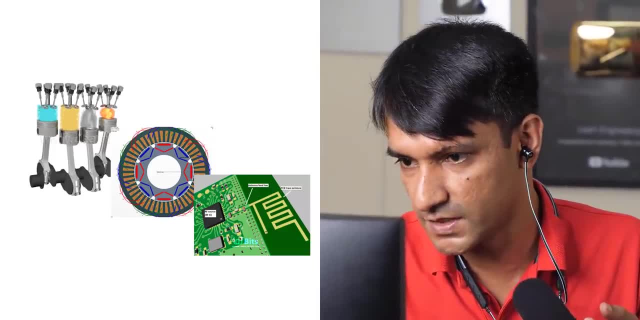 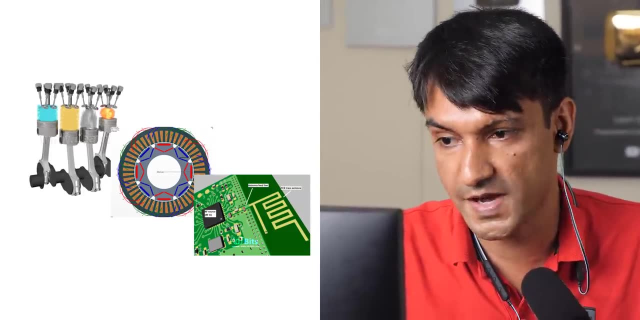 this electric motor. now it is having eight pairs of permanent magnets. I think it's an IPM synarum motor. instead of eight pairs of permanent magnets, we are using six pairs of permanent magnet. then how is performance will be affected, how the torque will vary, how the efficiency will? 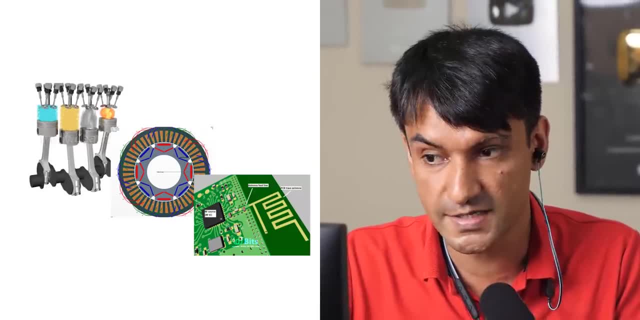 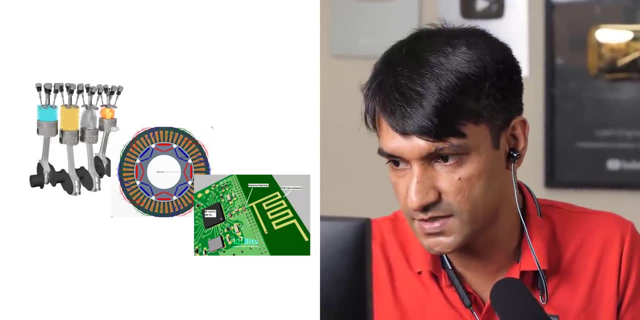 be affected. if we can give answer for this, if we can predict answer for that, then you are a good design engine for electrical machines or this antenna. now, this is the design of the antenna. instead of this design, if you are trying some other design- how the radiation patterns will be affected. if we can. 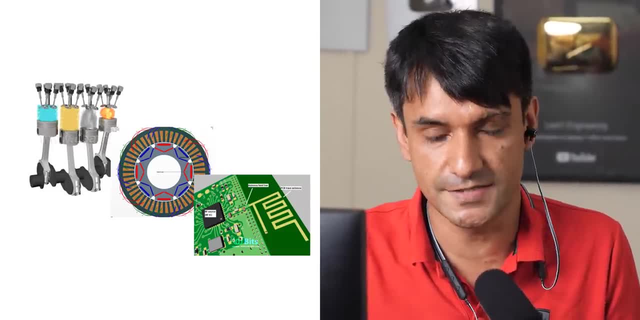 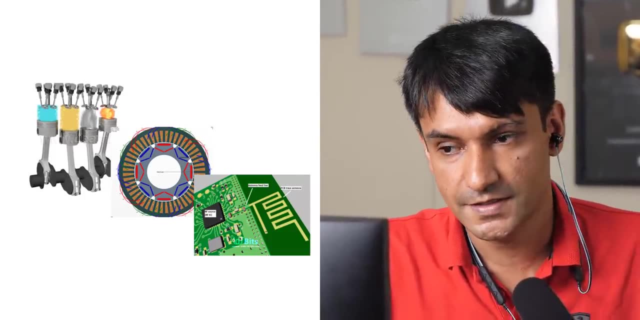 predict that you are a design. you are a good design engineer for antenna technology. so those who can predict the future will be able to predict the future. more specifically, predict the future of some technical thing. they can become a good design engineer. so, as we discussed earlier, to predict the future you need: 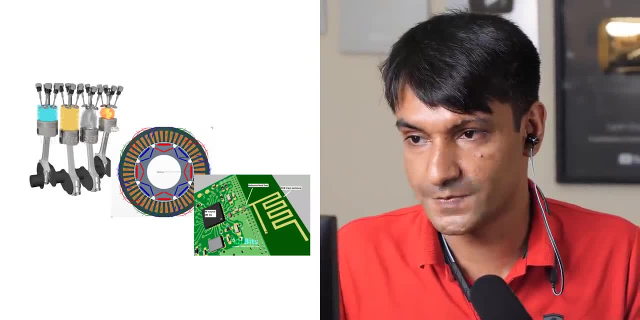 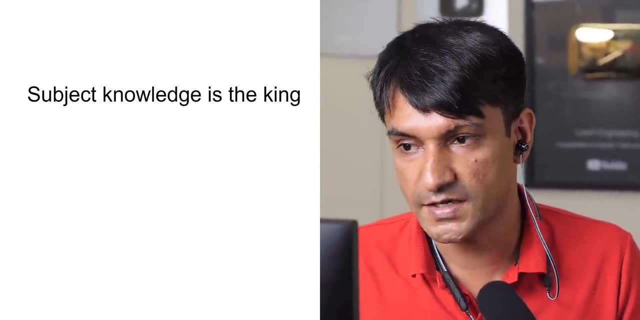 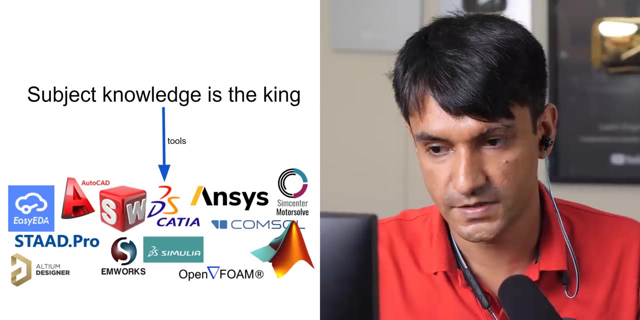 good subject knowledge? right, of course. subject knowledge is the king and nowadays you have a lot of software with you, lot of design software, analysis software and I will call them tools. your subject knowledge is the king and using all these tools, all this software, your life will be more easy and more. 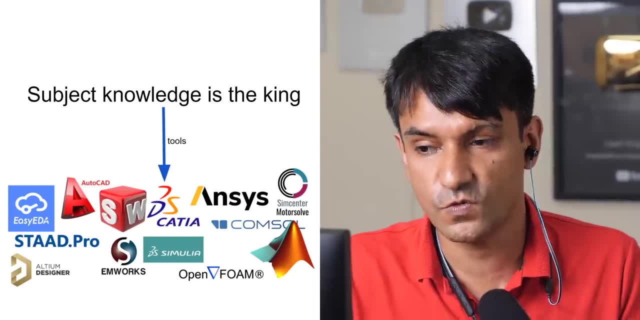 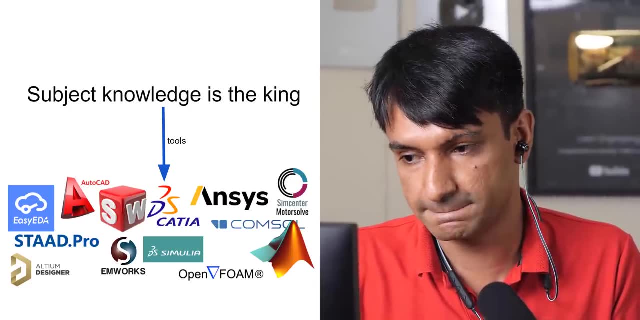 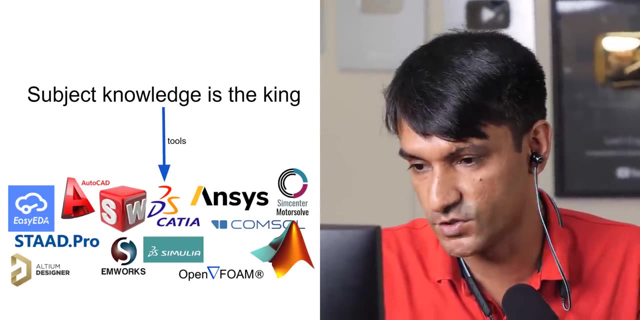 productive, and what I have listed here is a fraction of the software which is already available in the market. the actual number of software are maybe 10 times of this, and these are quite a fascinating thing if your subject knowledge is strong and if you know one of maybe three or four of these tools in 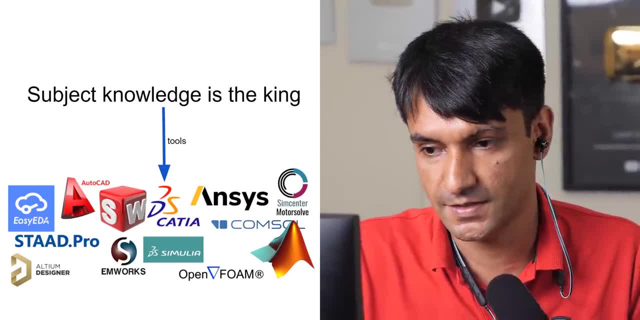 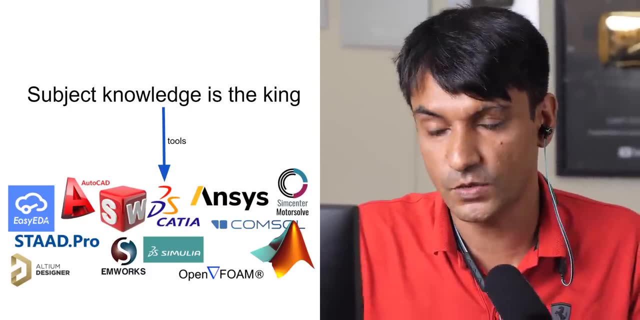 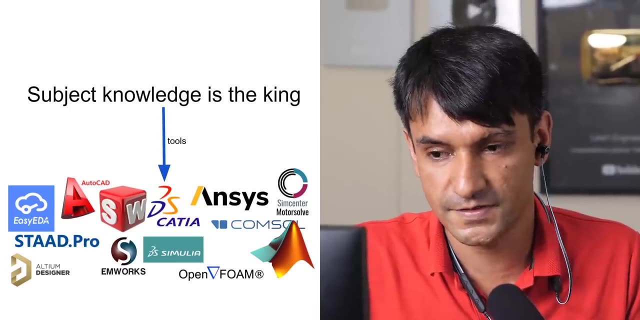 your domain and you are going to be very efficient design engineer. and if the reverse is the case, suppose you have, you don't have much subject knowledge, you know the software really well- then how that can be productive is like you have a car, there is a road, but you don't know how to drive is to be. 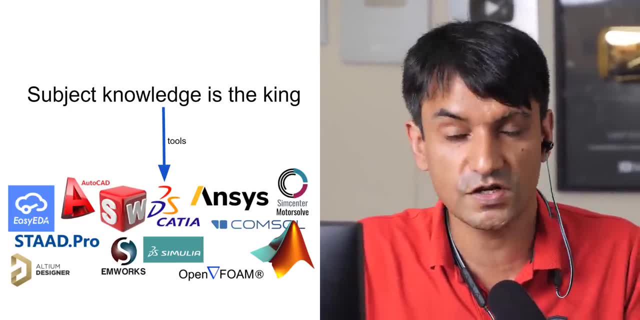 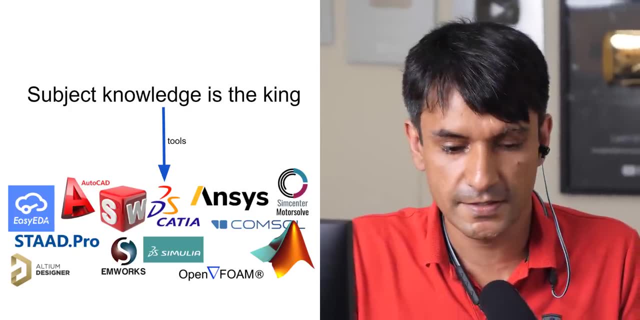 like that: you have the software, you know how to use it, but you don't have subject knowledge. it will be useless. maybe maximum you can make some CAD model, some drawing etc. but because all the software, even the espadrille simulation software, they'll throw out wonderful result, wonderful CFD or 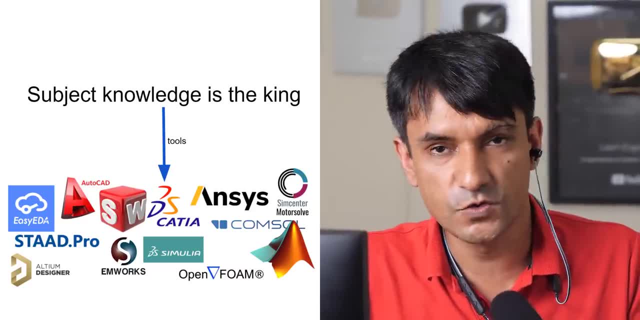 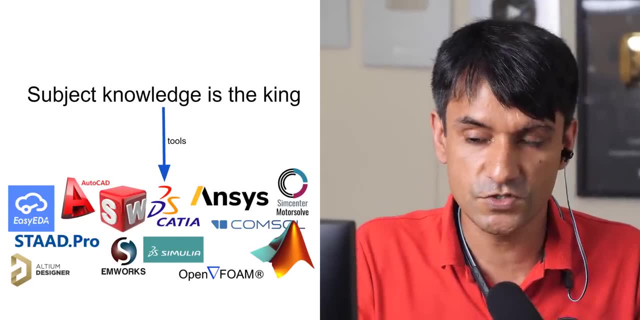 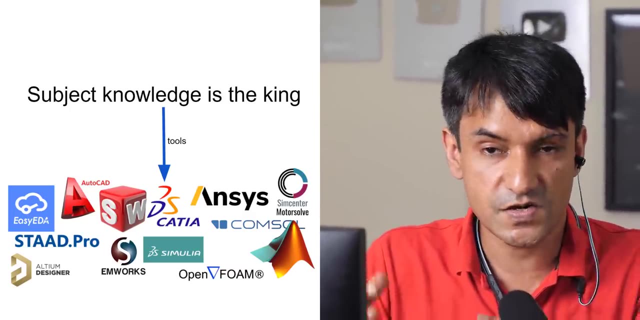 FCA result or system-based simulation. but how to predict these results are right? because this software are just machines, almost like machines. they can predict anything. is you to decide whether the results are right? was there any? was there any mistake in my software settings to predict whether results are right? you? 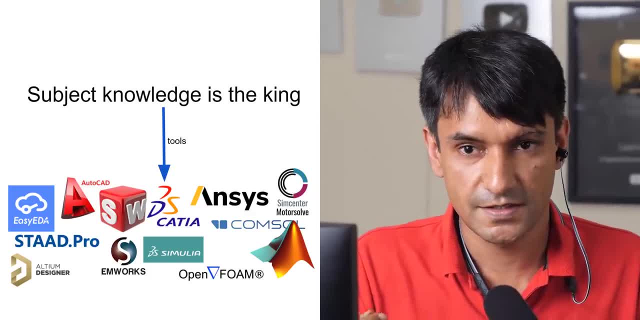 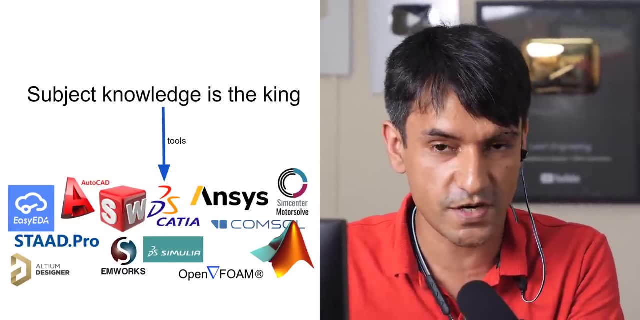 have to be good engineer with good subject knowledge and physics understanding. and even consider this scenario. suppose you got a result right, but the result was not fair enough to be a good design for that product. now you want to change the design, but how to have a proper judgment from that result? 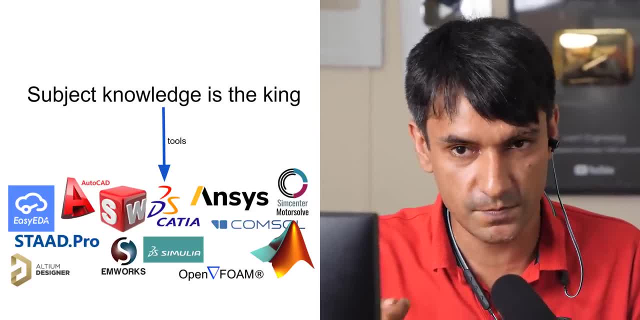 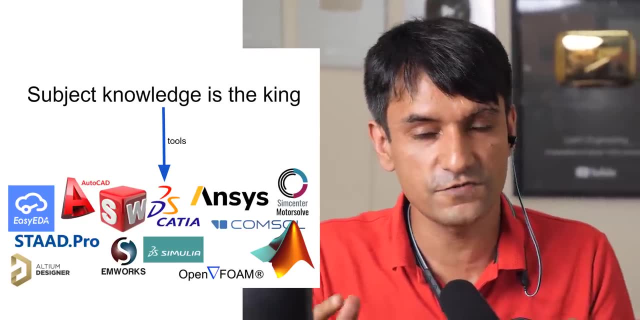 this is a design modification I have to do to improve my performance. so all these things are impossible if your subject knowledge is very weak. so my suggestion is that in your four years of engineering life, focus on improving your subject knowledge. focus on the fundamentals of the conceptual. 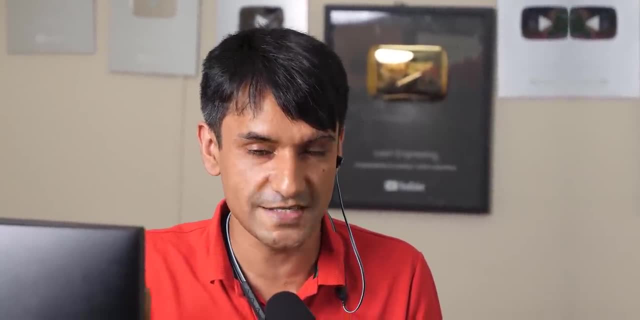 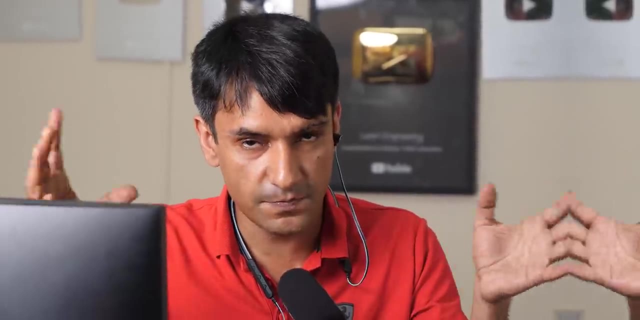 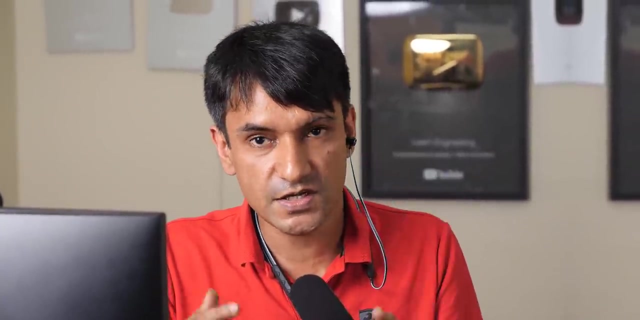 understanding. try to understand all the technology from the basis of physics, very deep level of understanding. that's really going to help you, because your test book might have some definite problems, but things are changing rapidly around the industrial world. people are coming with new ideas, new technologies. those technology might not have explain your test book, but if your physics is, 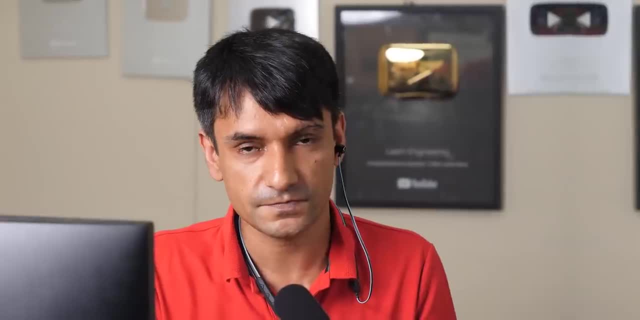 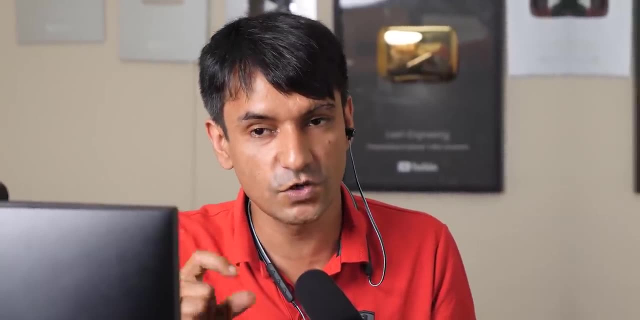 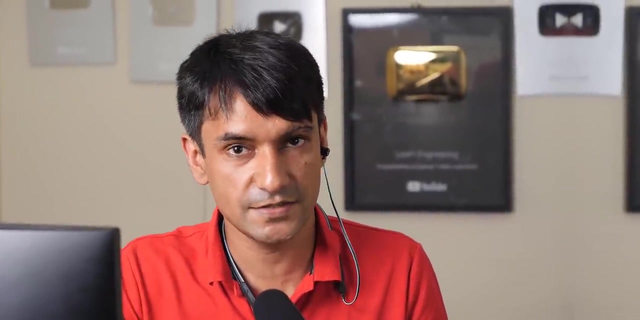 strong, you can easily predict, you can easily design them. also, if your mathematics is also strong, you can easily quantitatively predict how much will be the torque improvement my motor or what would be the new radiation pattern of the antenna, or what will be the torque variation of an IC engine. you can predict. 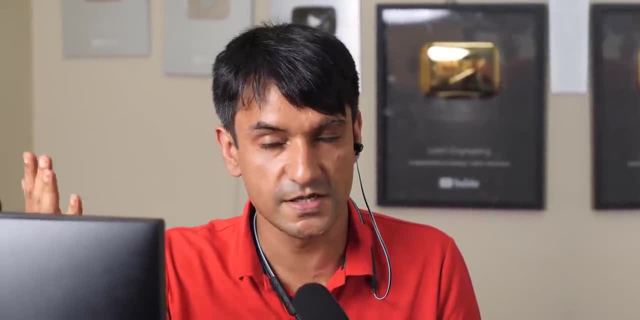 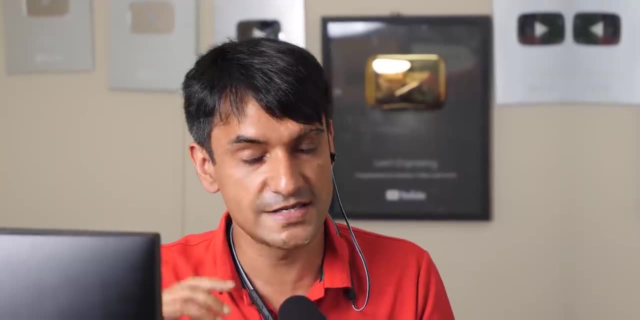 with proper values, this will be increased by five percentage. there will be reduction by by two percentage. if your mathematics is also good, based on your fundamental understanding, you can have analytical modeling and you can model them mathematically. so the mathematics you are learning, your engineering life is. 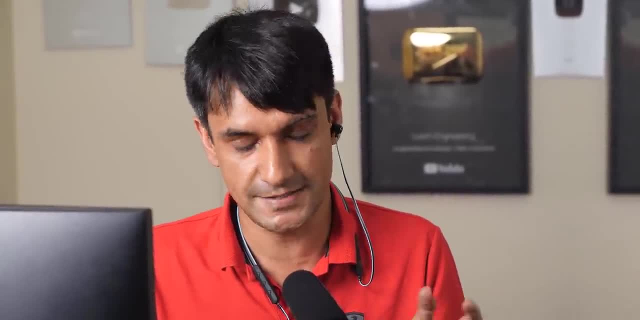 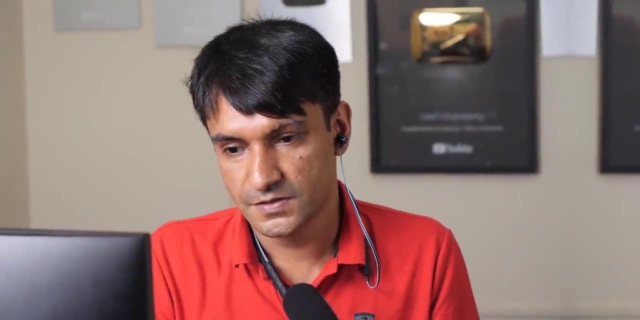 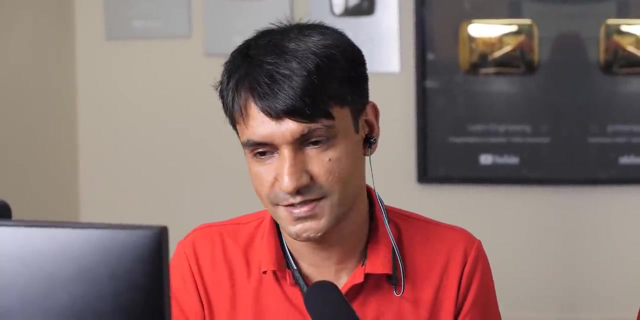 not useless. it's very, very helpful if you're a design engineer and obviously with all these tools, your life is going to be more easy. and nowadays the strength I can see in engineering colleges is that they take their subjects very casually, thinking that it's all about practical knowledge. it's all about 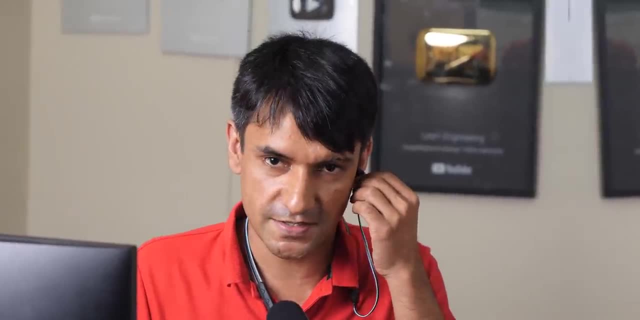 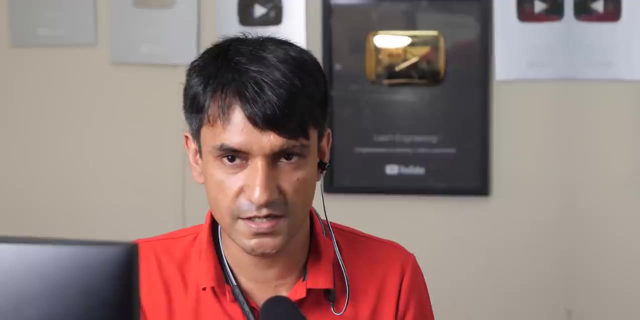 experience and software and I have interviewed many candidates. we have a design team here. we are doing some product development in my company. so for the recruitment I have recruited many candidates and some of them are like that: they know the software, they know SOLIDWORKS, they know ANSYS, but zero. 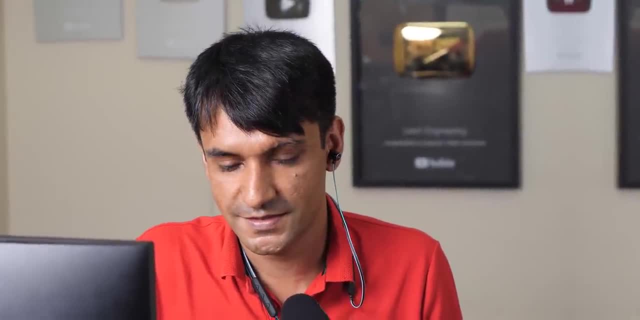 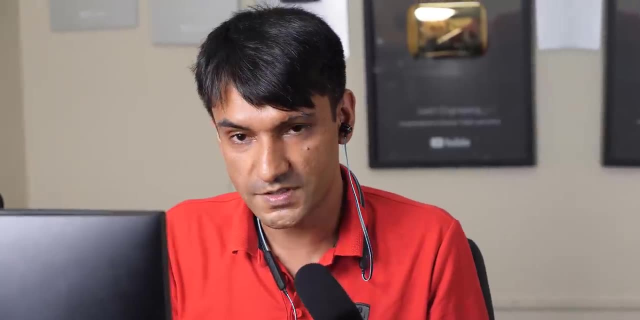 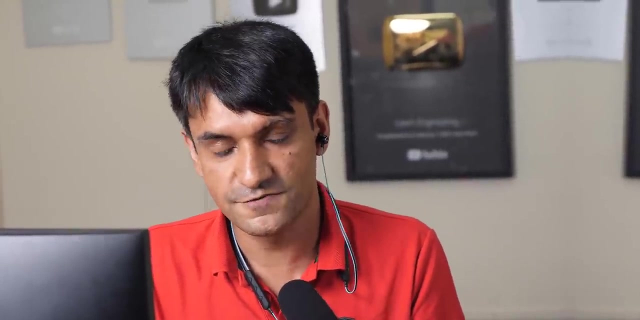 subject knowledge, then what's the point? they won't be able to use it, they won't be able to make any proper judgment from the result. so don't get trapped with this, don't get trapped in this false advices. subject knowledge is always the key, in fact, the duty of your engineering colleges. in four years of. 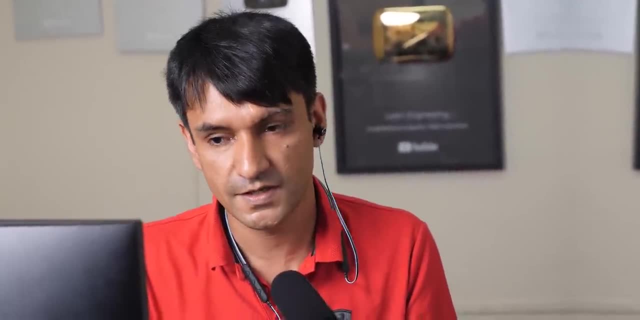 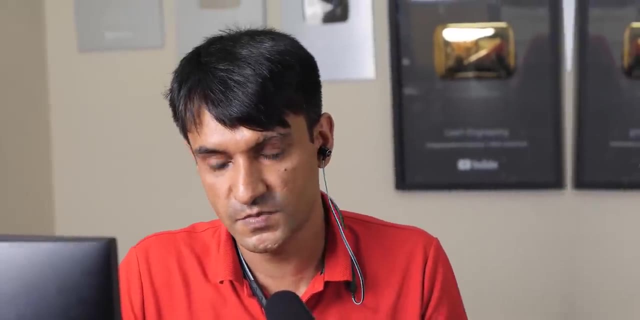 engineering life is to transfer the subject knowledge properly and learn the software. to make them learn the software is not their duty, is your duty. you have to learn it because number of the software are infinite. there could be more than hundred such software. so if your engineering college cannot, 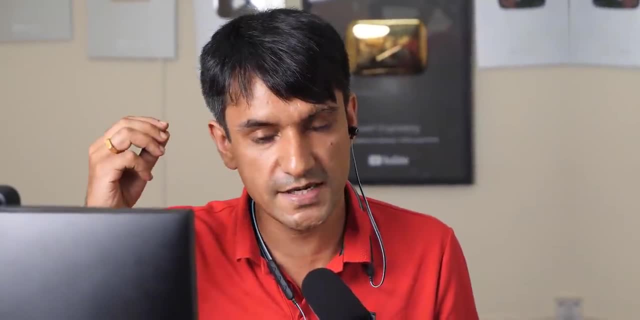 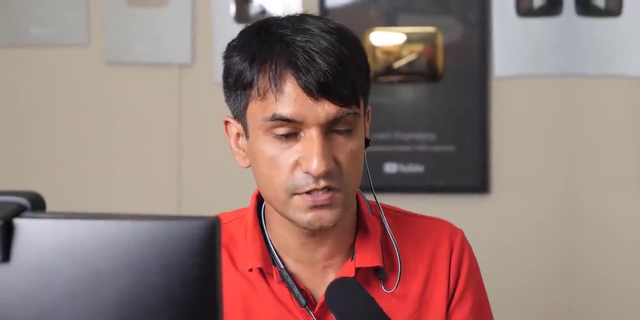 teach all this software. it's your duty. you have to decide which area you have to focus. you cannot focus on the all the areas of a branch. even if you are mechanical engineer, you can focus on all the design departments. you have to decide. this is my area of specialization. 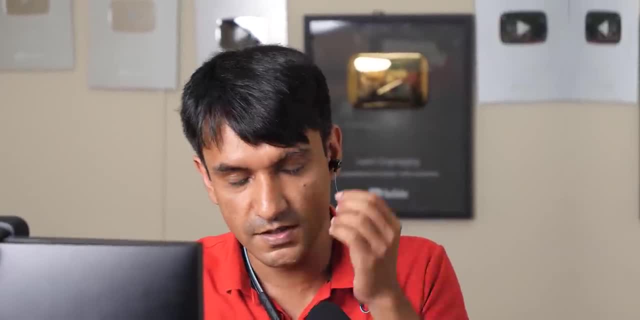 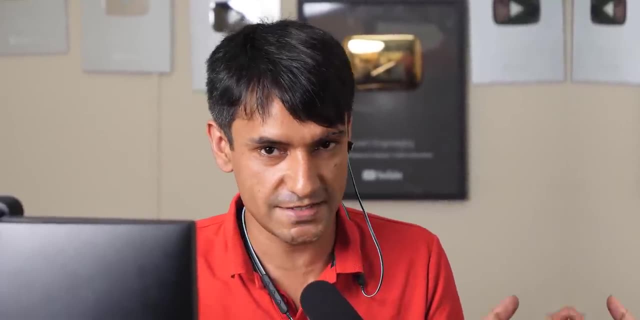 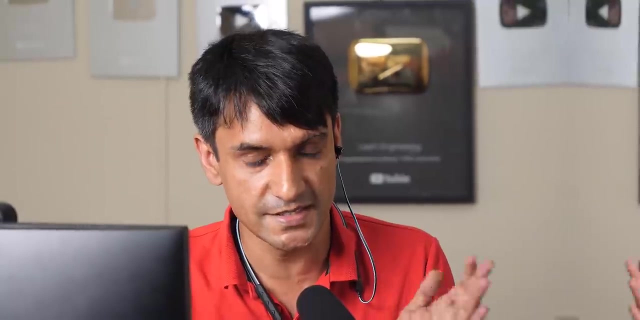 mechanical engineering and learn three or four sub software. also focus on subject of, focus on fundamentals of the subjects. learn it really well, then you will be a deadly combination. all the companies will want to recruit you. with proper subject knowledge and proper software knowledge, you will be a perfect and amazing.